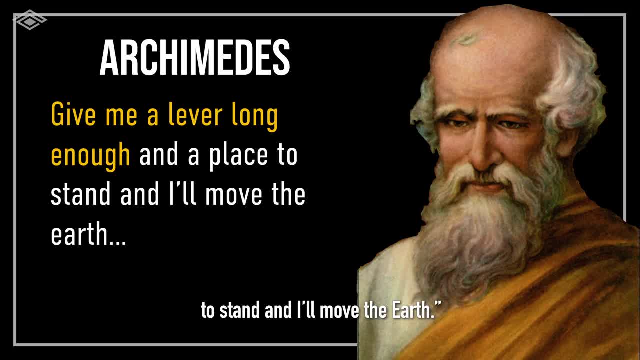 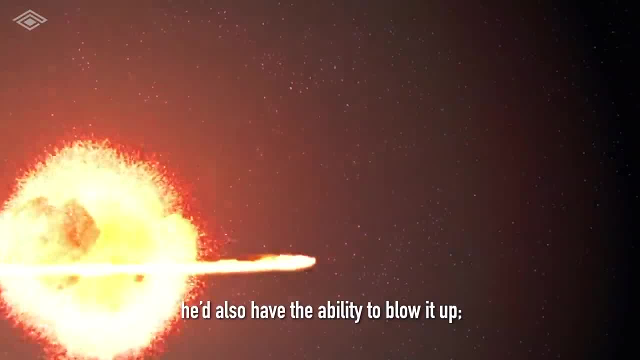 Archimedes once said: give me a lever long enough and a place to stand, and I'll move the earth. If he was standing in something more sophisticated like the Death Star, he'd also have the ability to blow it up, if he knew how to operate it. of course, In the 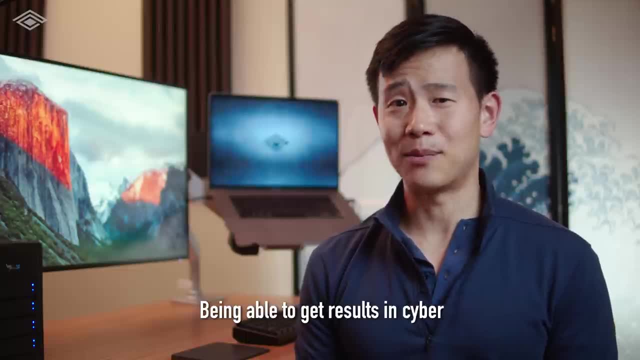 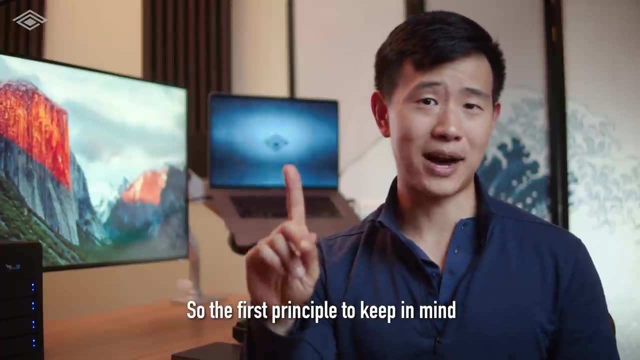 cyber world it's no different. Being able to get results in cyber depends on the types of software tooling at your disposal and your expertise at using them. So the first principle to keep in mind is that it's the combination of tools and skills that really determine your overall cyber abilities, whether 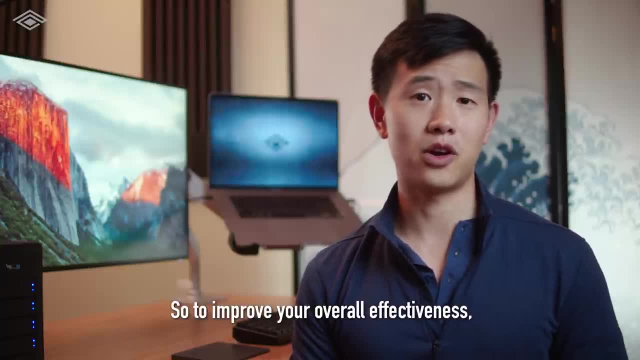 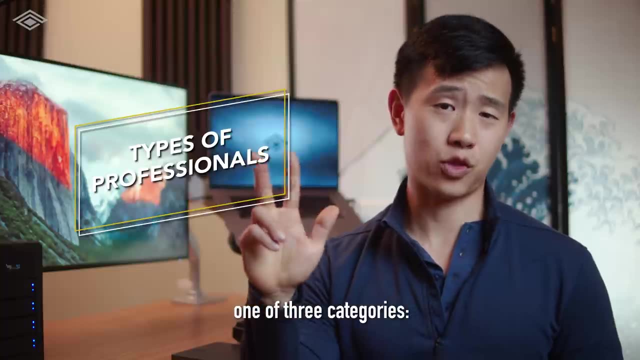 for an individual or for a team, So to improve your overall effectiveness, it's important to be balanced in both. Currently, in the field of cybersecurity, most people fall into one of three categories: black box users, tool operators and developers. 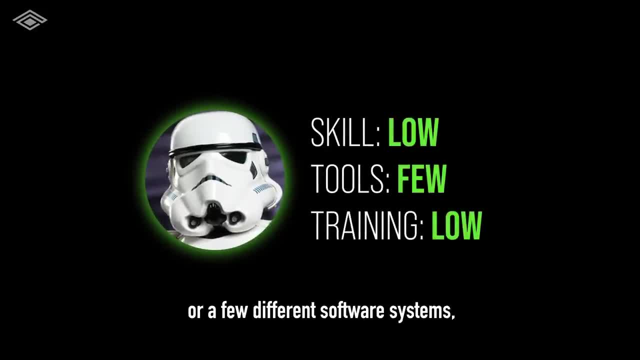 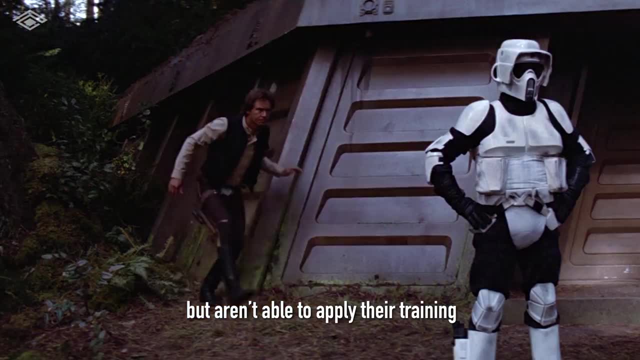 Black box users will usually only know the basics of using one or a few different software systems, and only in situations that they've been trained in. These guys might even have a few certifications, but aren't able to apply their training to solve problems independently. 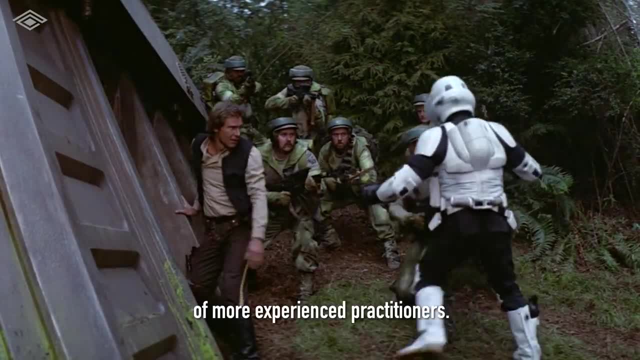 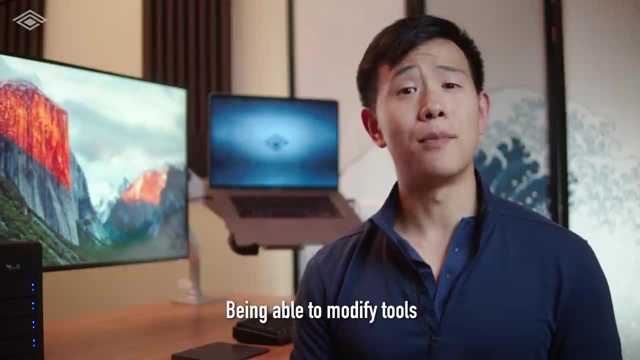